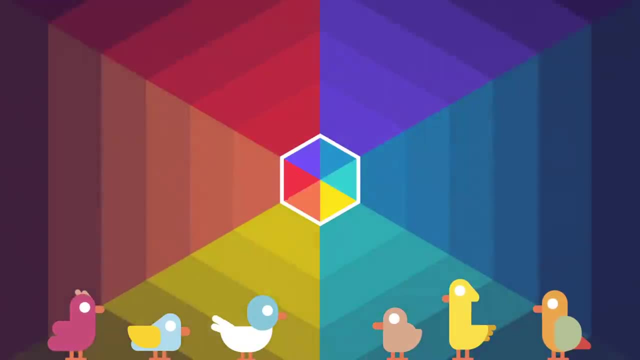 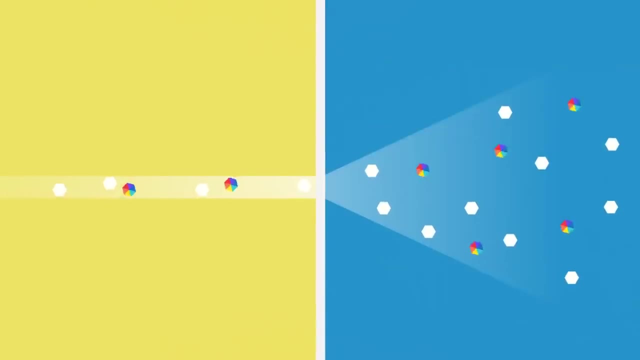 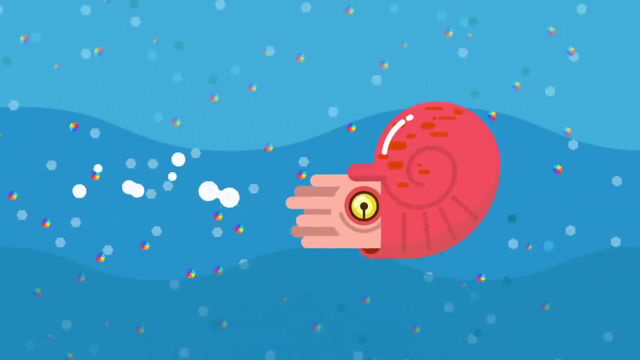 We just happen to have evolved eyes that are good at registering exactly this part of the electromagnetic spectrum. This is not a complete coincidence, though. Light is the only set of electromagnetic radiation that propagates well in water, which happens to be where most eyes first evolved, millions of years ago. 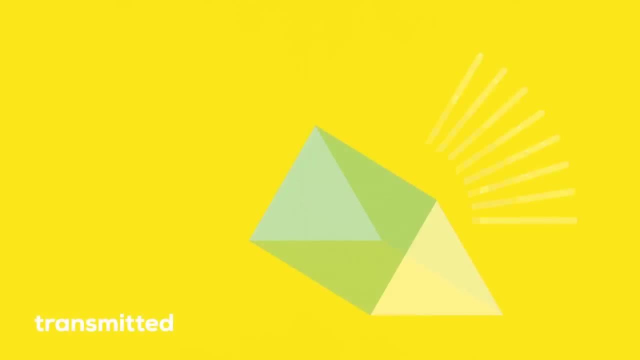 That was a smart move, because light not only interacts with matter, it's also altered by it and can be used to gather information about the world around us with almost no delay, which is arguably really helpful for survival. Okay, where does light come from? 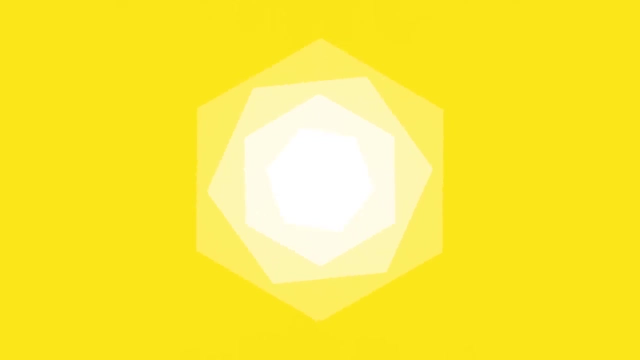 A vast range of electromagnetic waves are created when atoms or molecules drop from a higher state of energy to a lower one. They lose energy and emit it in the form of radiation. At the microscopic level, visible light is created when an electron within an atom. 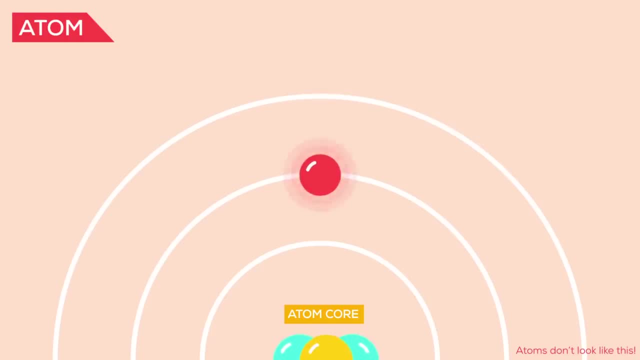 that is in an excited state drops to a lower energy state and loses this excess energy. The same way, incoming light can elevate an electron to a higher state of energy by being absorbed by it Macroscopically. the moving charge of the electron creates an oscillating magnet field. 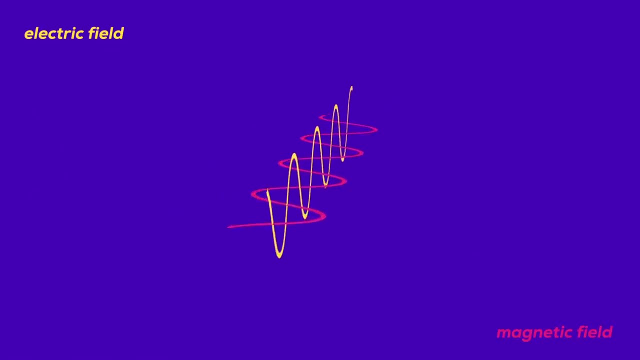 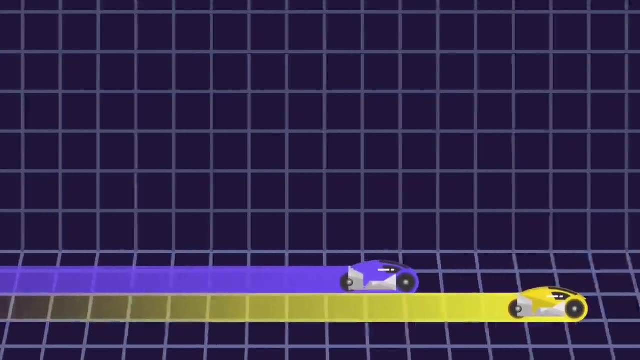 which creates an oscillating electric field perpendicular to it. These two fields move themselves through space, transferring energy from one place to another, carrying information about its place of creation with it. Why, of all the things in the universe, is light the fastest thing there is? 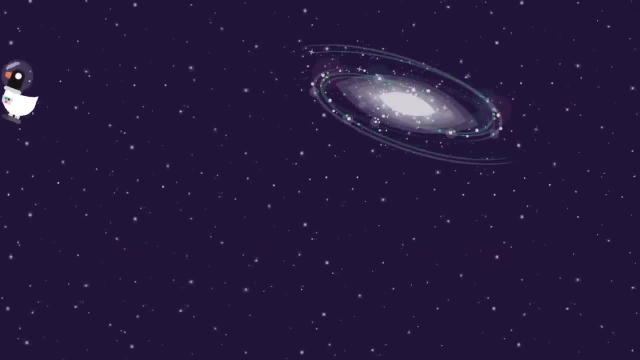 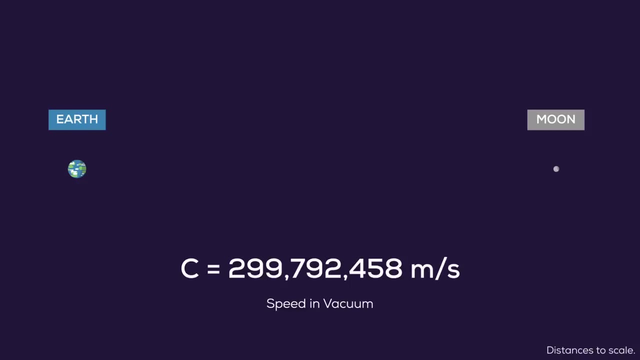 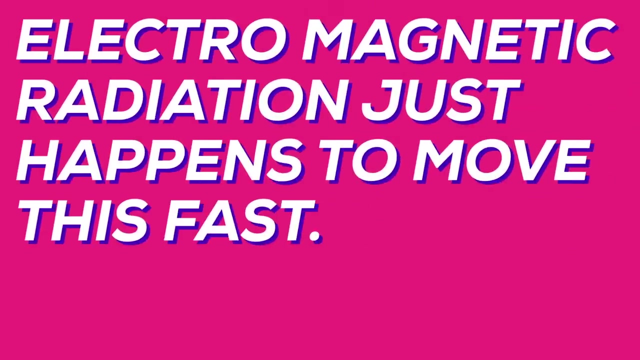 Let's change the question: What is the fastest way to travel through space in the universe? It's C Exactly 299,792,458 meters per second in a vacuum. One billion kilometers per hour. Electromagnetic radiation just happens to move this fast. 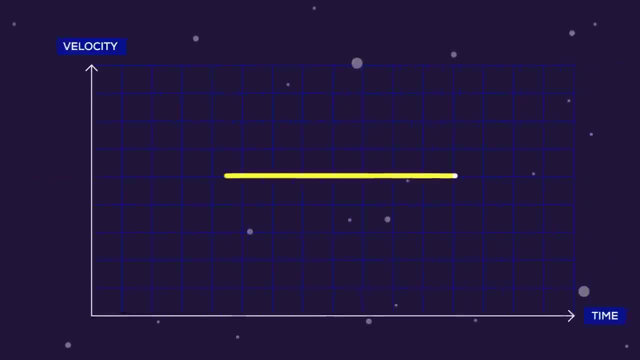 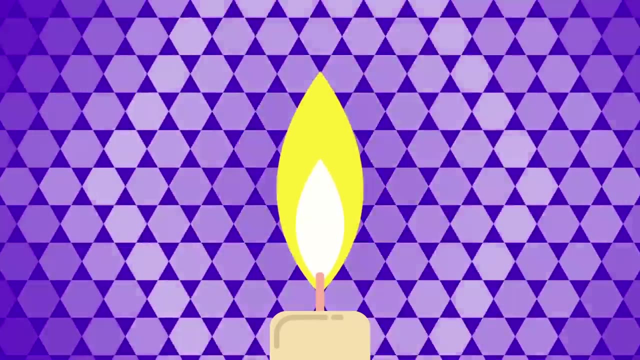 Any particle that has no mass travels at C without acceleration or any in between. The light that's being released from a candle does not speed up until it reaches light speed. At the very instant of its creation, its speed is C. So why is C, or the speed of light, finite then? 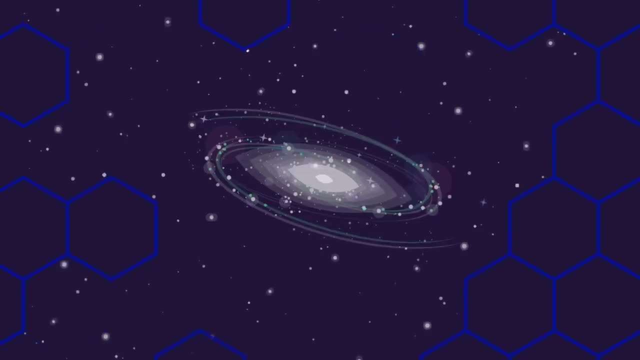 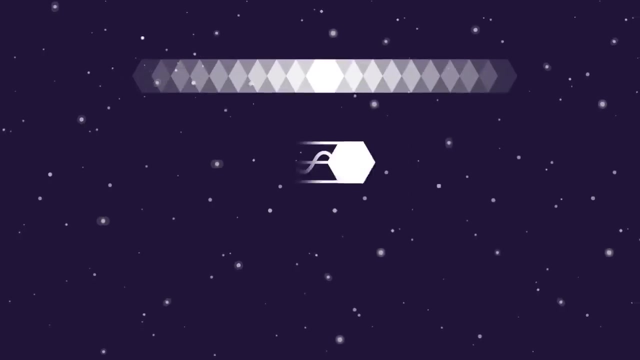 Well, nobody knows. Our universe is just built this way. We don't have a smart answer here. So light is a part of a spectrum, a planetary particle that also behaves like a wave, propelled by two perpendicular fields, traveling at the speed limit of the universe.